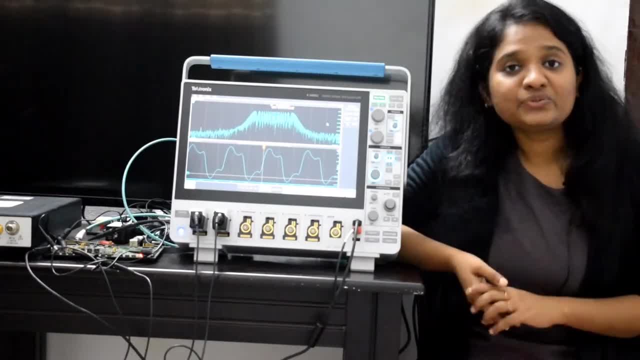 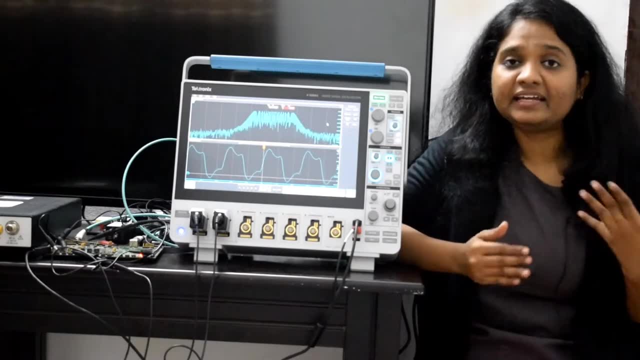 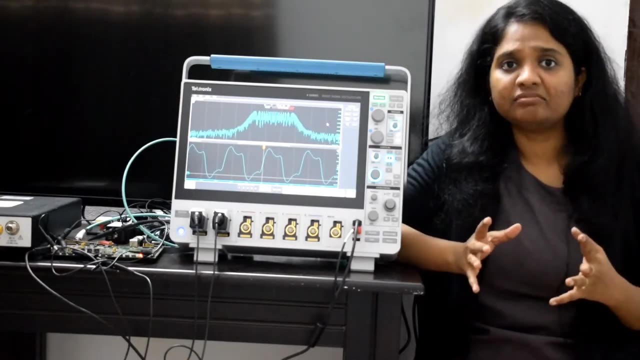 Looking into the time domain. representation of your signal using an oscilloscope may not reveal the full information of your signal and most of the engineers again go to the spectrum analyzers to see the frequency content of your signal. This is true when there are some noise, that is. 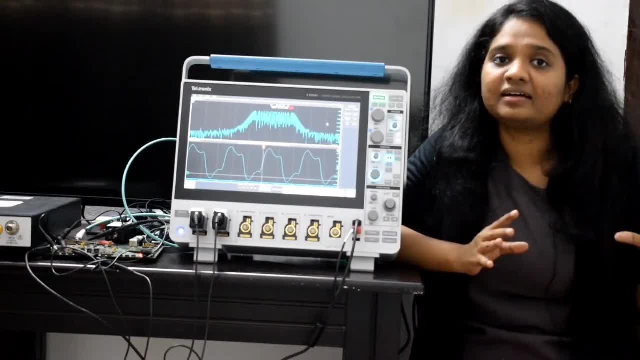 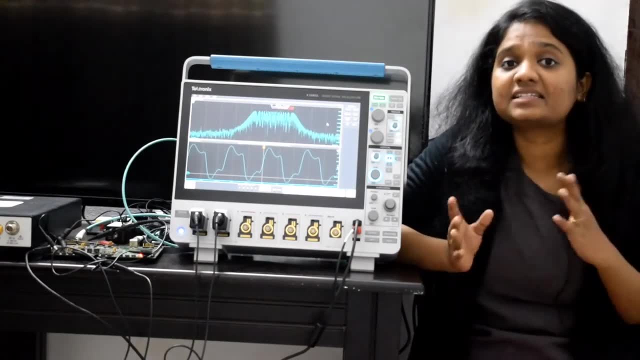 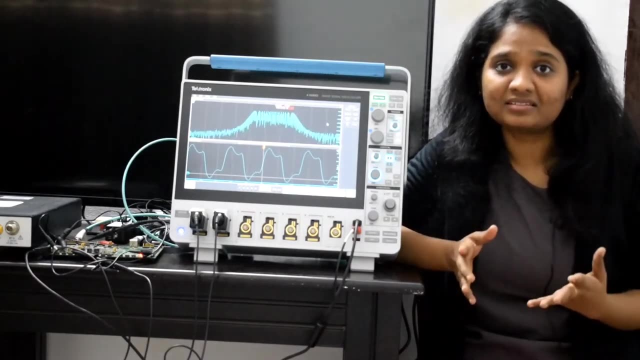 present in your time domain waveform. but you need to understand what causes that noise. what are the frequency components or any modulations as present in your signal that is creating this behavior in time domain? Hi, this is Neetu. Today I'm going to show you how to do the spectrum analysis using 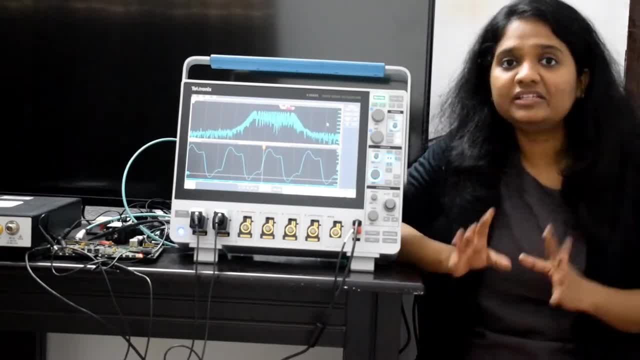 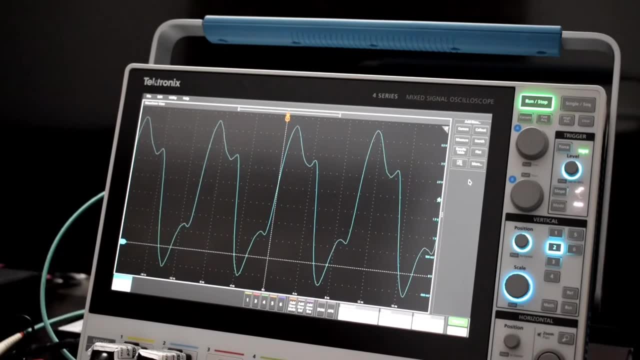 oscilloscope and how the DDC based spectrum view is different compared to the math based scope, FFT. Today we are using Tektronix 4 series MSO, which is having digital down converter built into it hardware and I'm having a clock signal. 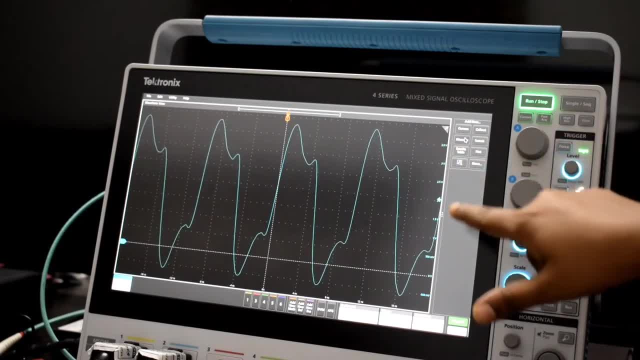 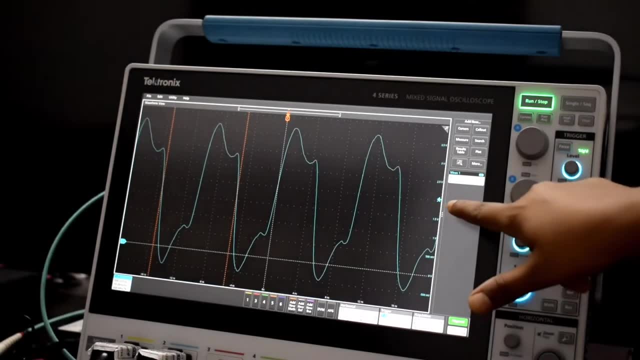 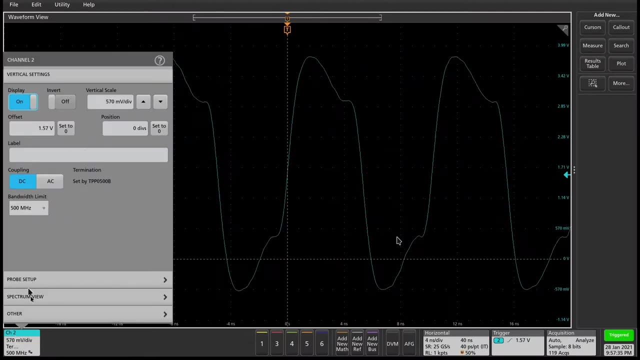 First, I want to measure the frequency of the signal. I'm adding the automatic measurement, which shows the frequency of the signal as around 98 megahertz. It's pretty easy to set it up: I just need to go to the channel settings and. 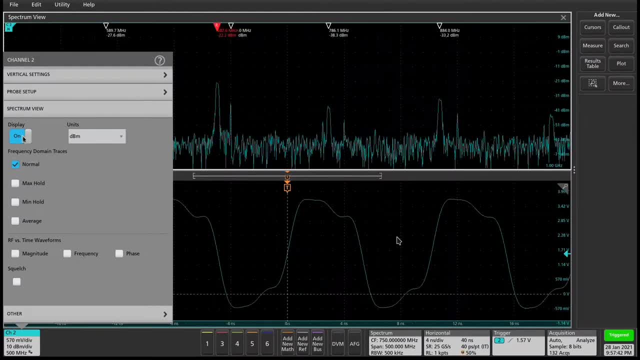 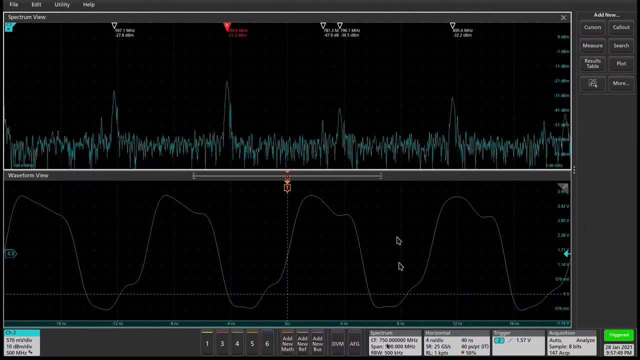 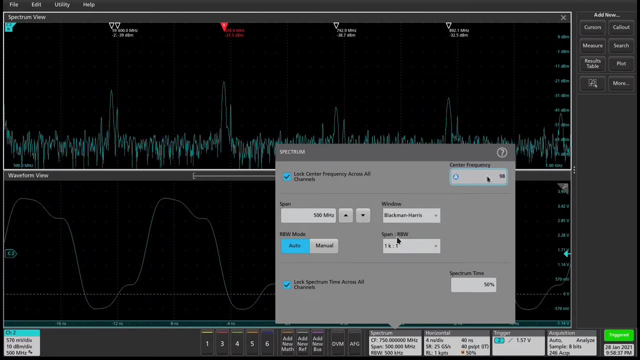 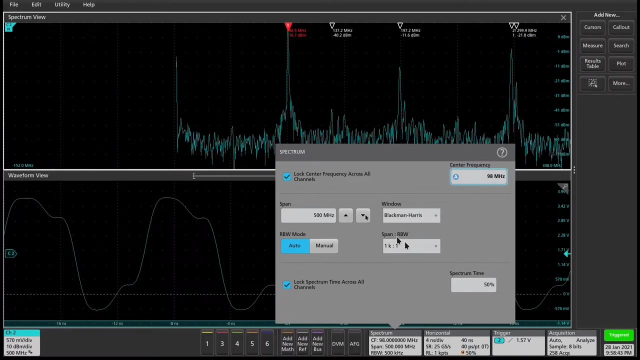 turn on the spectrum view. Now I got both the time and frequency domain view of my signal. Let's configure the spectrum by going to the spectrum view controls. Here I have all the settings that are similar to a spectrum analyzer and I'm going to adjust my center frequency to 98 megahertz, which I've measured and 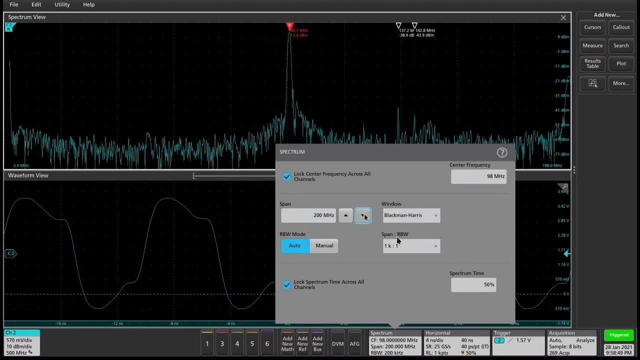 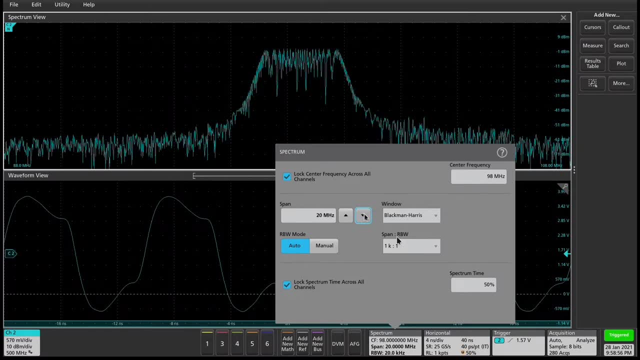 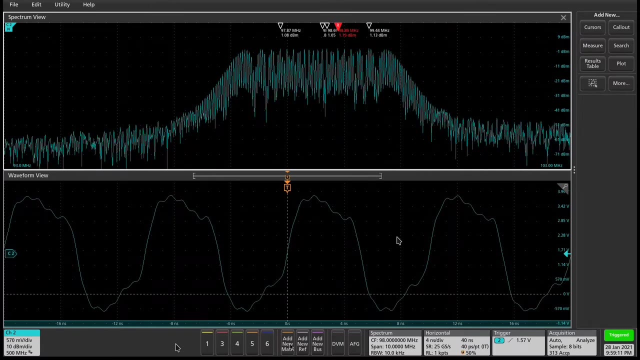 adjusting my span so that I get a clear view of my signal. So now I set the span to 10 megahertz to see the spread spectral behavior of my clock. Now let's take a look at how we can do the same using math: FFT. 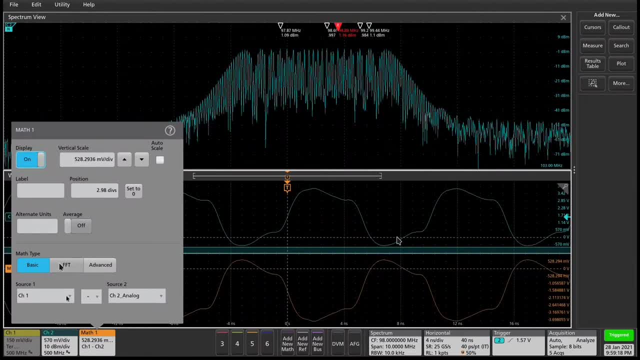 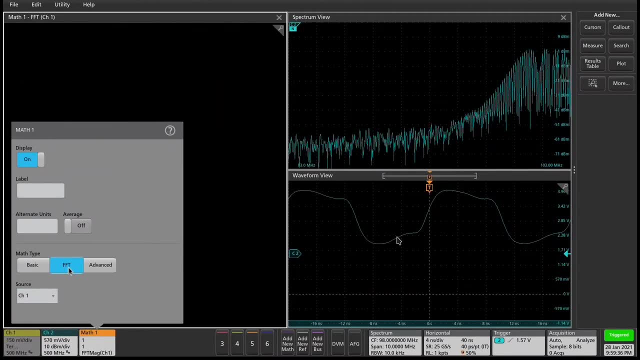 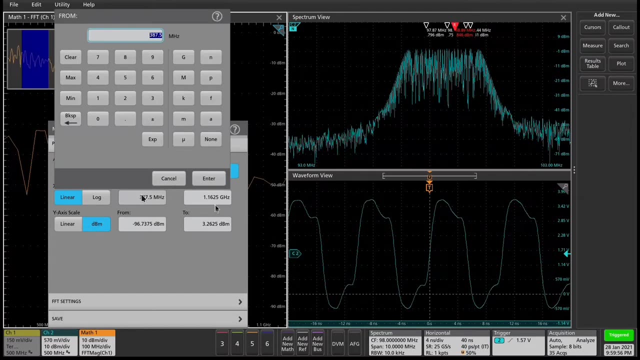 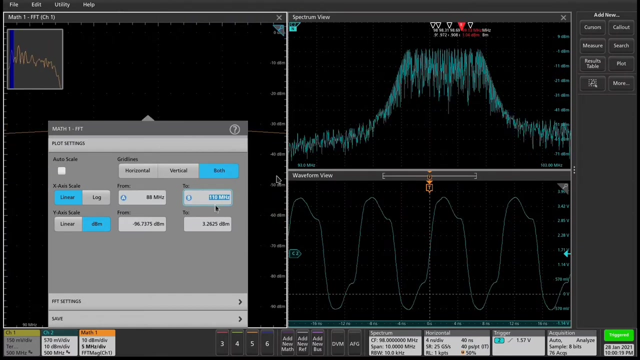 For that. I'm adding the math channel and adjusting the source to my current clock source, which is channel 2, and enabling the FFT. Here I'm adjusting the start and stop frequency of my FFT to match it to my spectrum view. Now I'm going to set the time domain view to 98 megahertz and I'm going to set it to 98 megahertz.